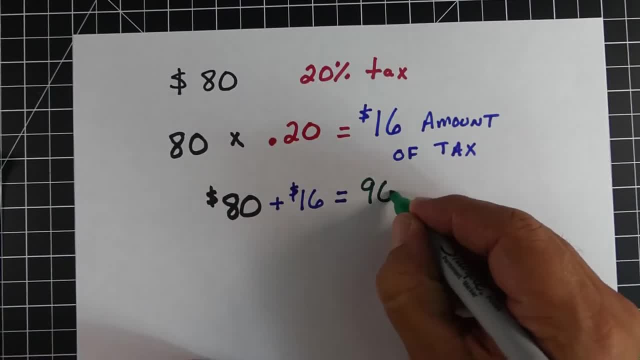 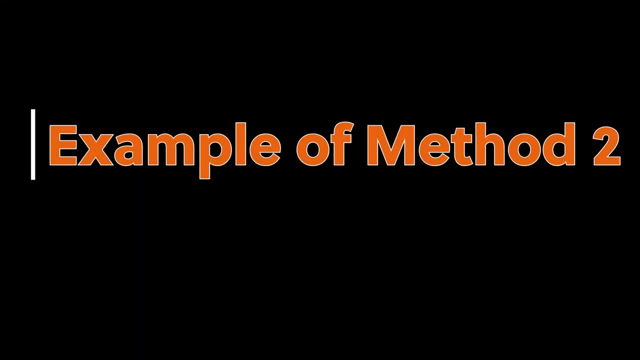 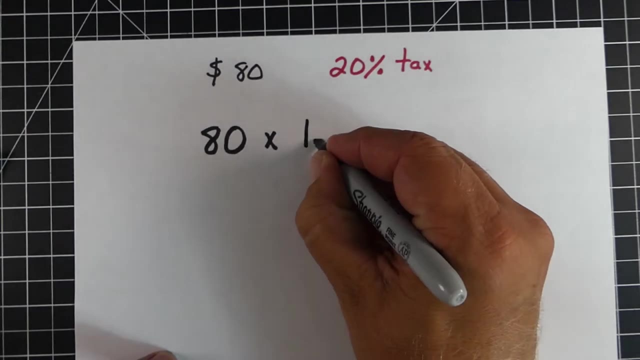 which is the total amount plus the amount of tax, which is $16., And that gives us our total cost of $96 with tax. Now here's an example of method two. So we're going to use the same amount, the same situation: $80, 20% tax. What we're going to do now is we're going to take the $80. 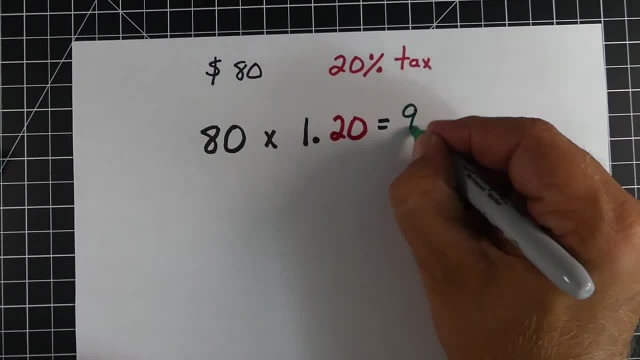 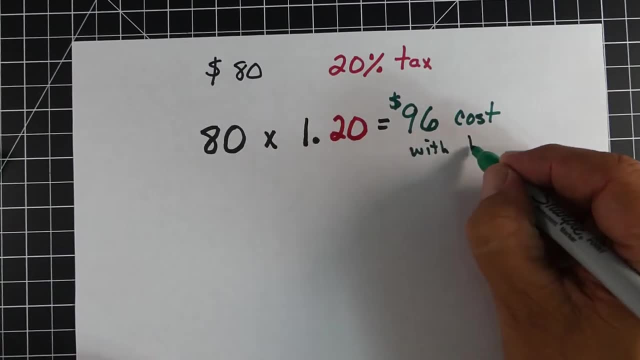 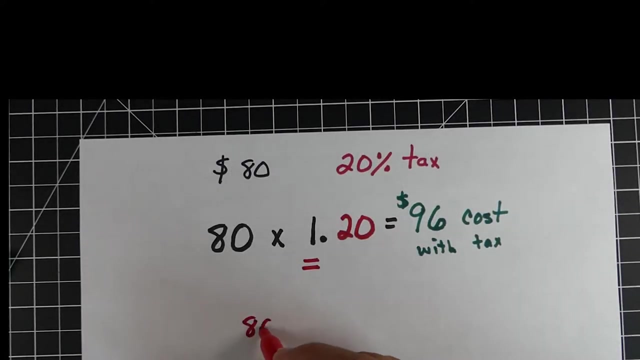 and we're going to multiply by 1.2 or 1.20. And when we do that, we also get $96. So we actually get the cost with the tax doing it this way as well. Now you might ask yourself how is this possible? So, if you want to think of it this way, 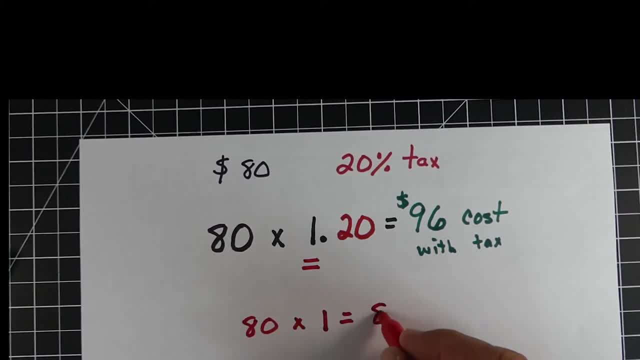 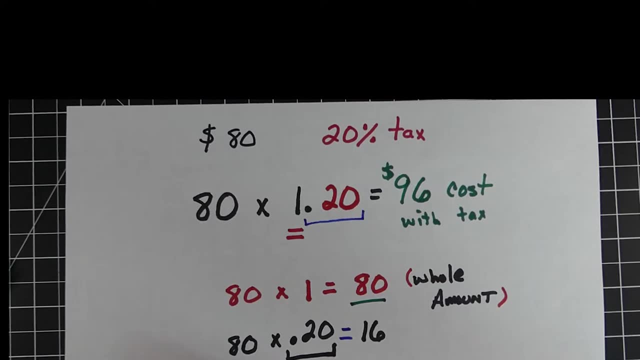 we know that 80 times 1 would be $80, or the whole amount, And we already know that we can take 80 times 0.2 and get the 16, which was the amount of tax. So what we can do is if we just combine the 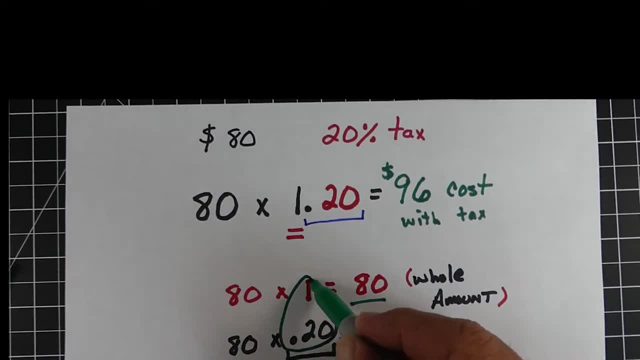 two, the 1 and the 0.2, we can get the $86.. And we can also take the $80 and the 1.2 and the 1.2 that's going to equal that 1.2.. So basically we're just taking the whole amount plus the. 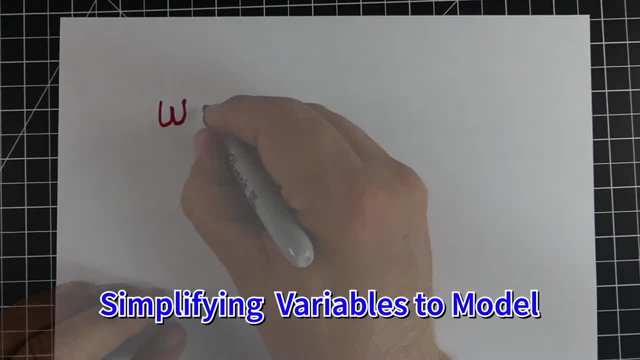 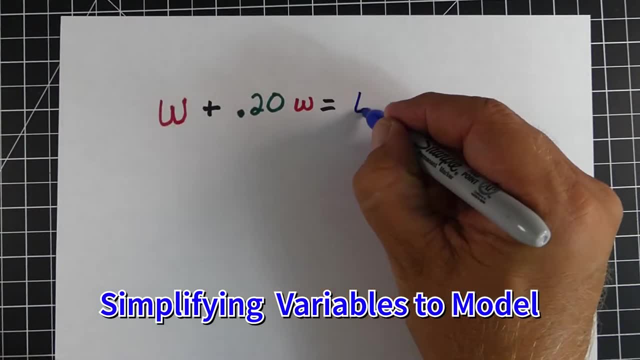 percent of tax and putting it together Again. you can think of this as a variable too, So the whole amount would be like a W or a 1W, And the amount of tax was 20% or 0.2W. So if we combined, 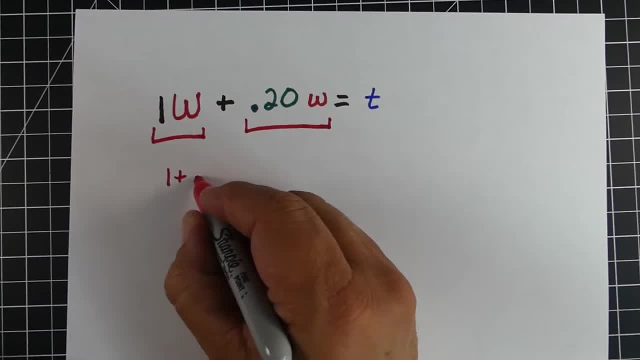 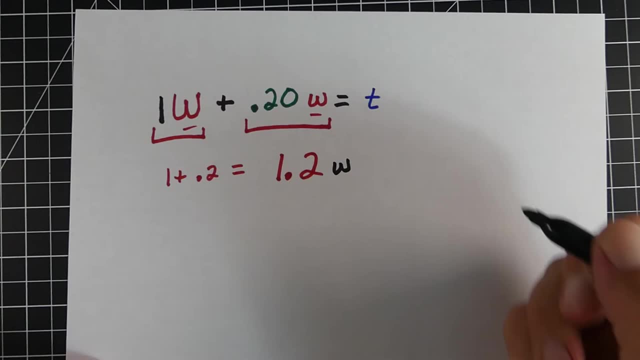 these two Ws, like we combine our common variable, we would take the 1 plus the 0.2, and we get 1.2W And that's going to equal our total. So 1.2W equals T. 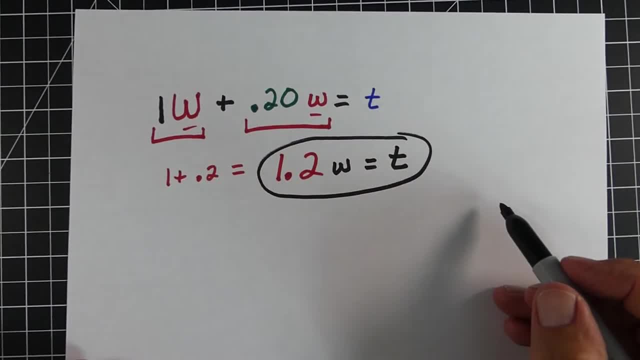 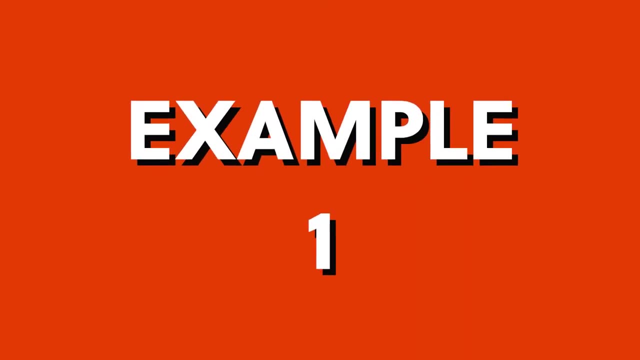 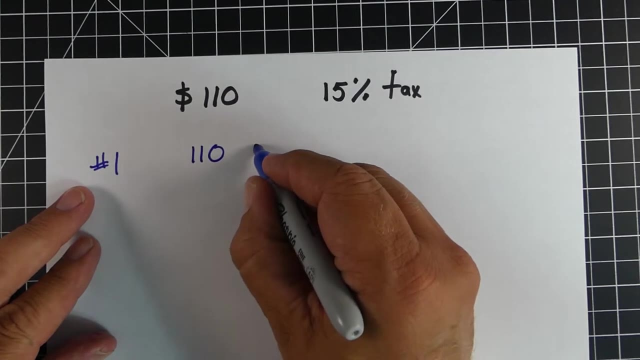 And so that's how we could kind of set this up as an equation. Now here are three examples, and we're going to use both methods in each of these. So here's example number one: All right, we have $110 item with 15% tax. So using method number one, 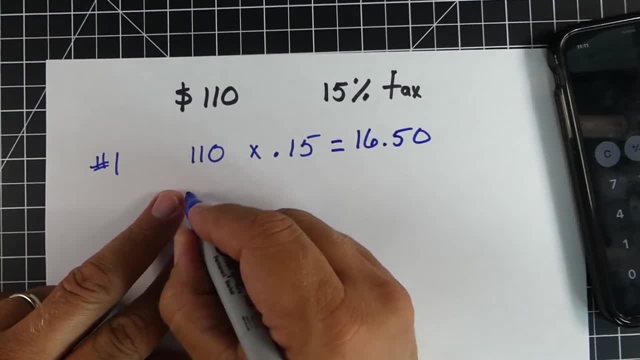 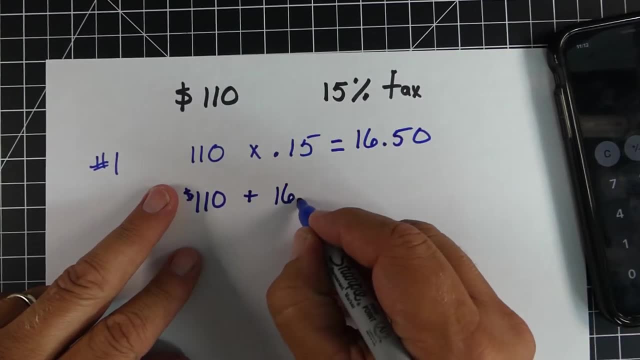 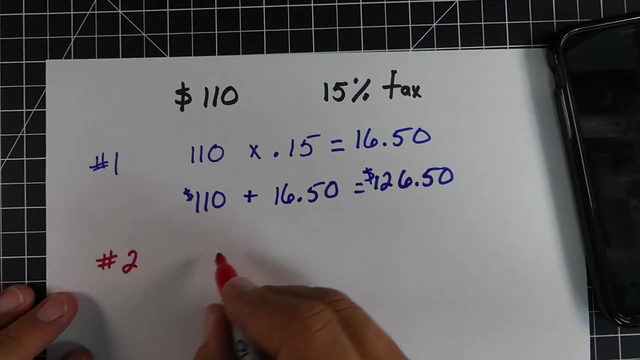 we take our total cost $110.. We multiply it by the decimal 15%, which is 0.15,, and we would get $16.50.. We're going to take that $16.50, which is the tax, add it to the original amount $110, and we get $126.50.. Now method two. 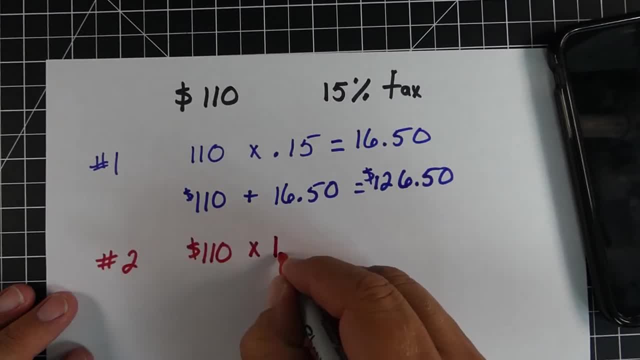 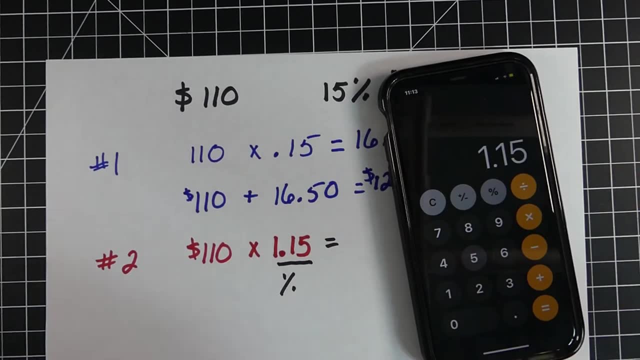 we would just take the $110, and we're going to multiply it by 1.15.. So that's the whole amount and the 15% tax. So if we multiply those two together, you can see that we're going to end. 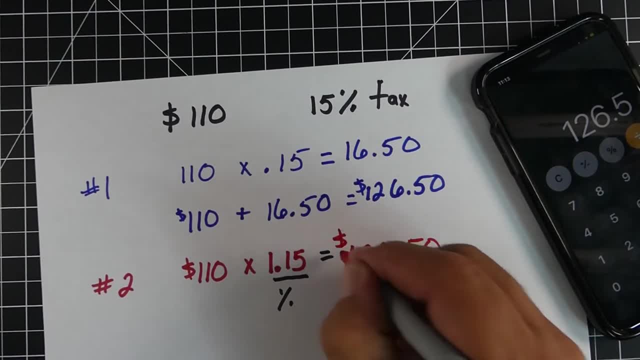 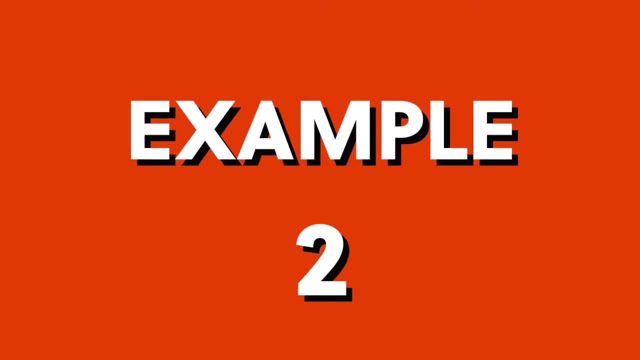 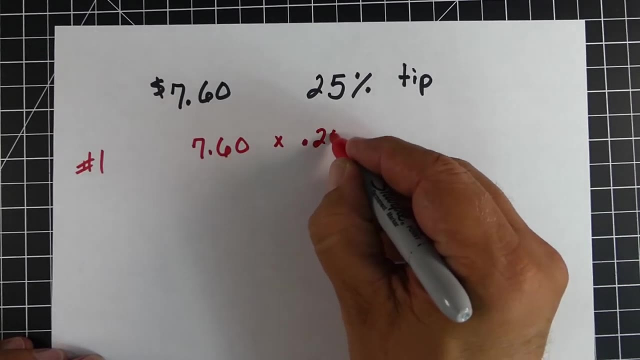 up getting the same amount: $126.. So both ways we're going to end up with the same answer. So here's example number two. So in this example we have a $7.60 meal and we decide we're going to leave a 25% tip. So you can. 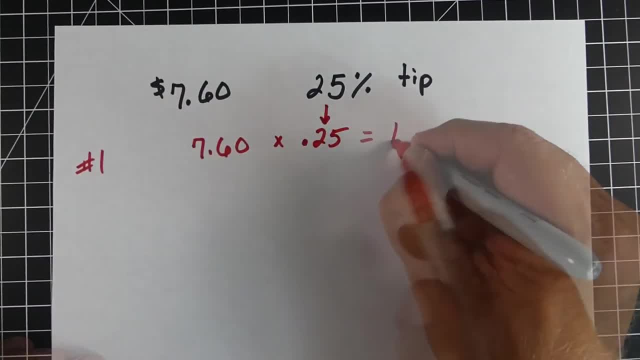 see, we're taking 760 times 0.25, which is 25% written as a decimal, and we get $1.90.. Now this $1.90, this is going to represent the amount of tip that we're going to leave for the waiter. 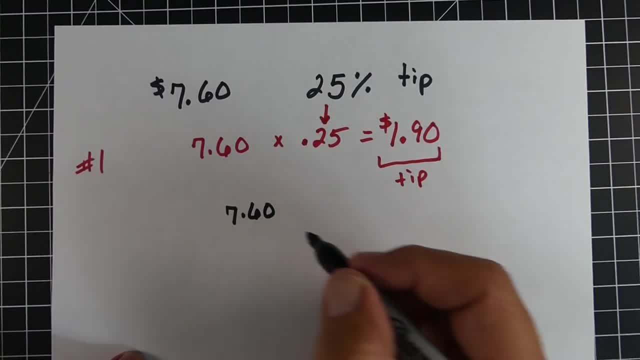 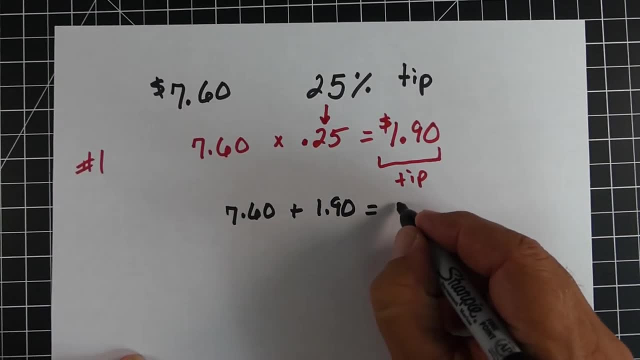 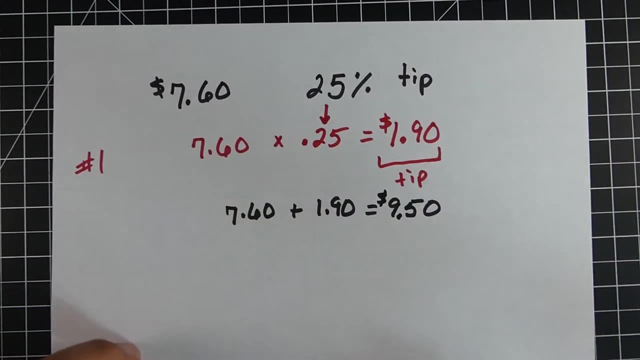 or the waitress. So in this first method, we would take the total cost of the meal, which is 760, and we're going to add the amount of tip that we're going to leave for the waiter or waitress, And so when we do that, we end up with $9.50.. Now, if we were to use method two, we would 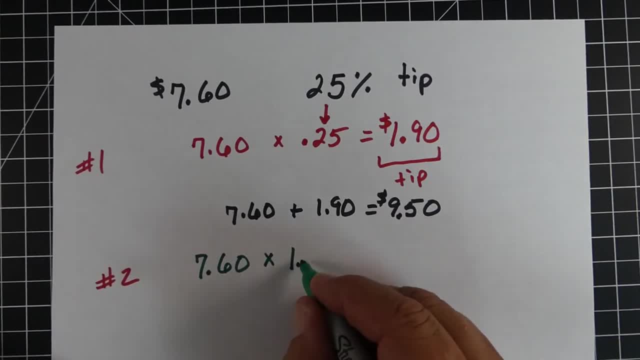 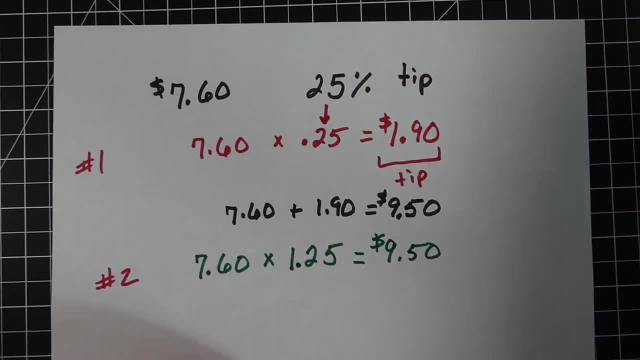 take the 760 from the meal and we're going to end up multiplying that by 1.25.. The one's the whole amount, the 0.25 is the percent of tip And we end up with the exact same answer. 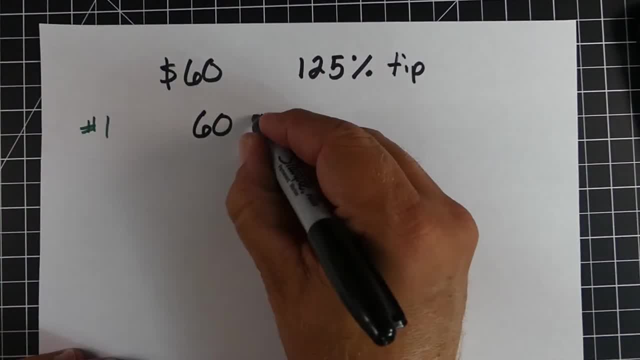 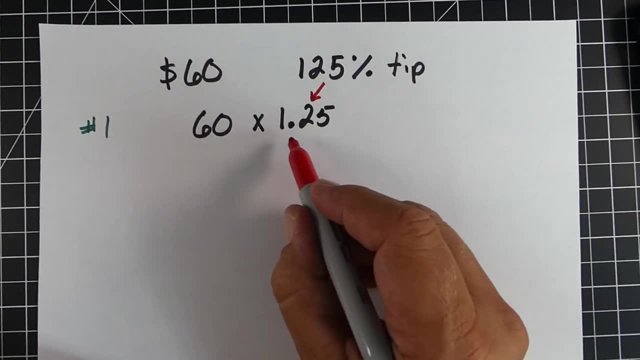 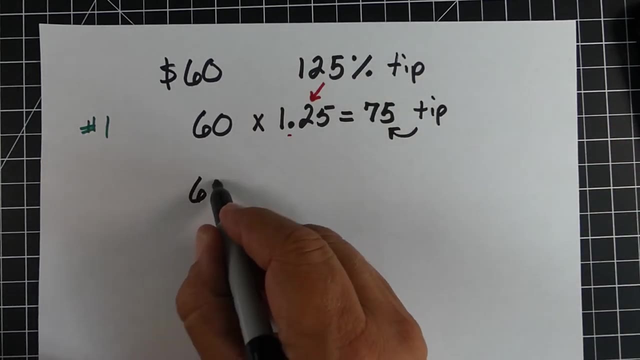 All right. on our third and final example, we're back at the restaurant and this time we're going to leave 125% tip on the $60 meal, So very, very generous. So, using method one, we take the $60 times 1.25, and we get our $75,, which is the amount of tip. That's quite. 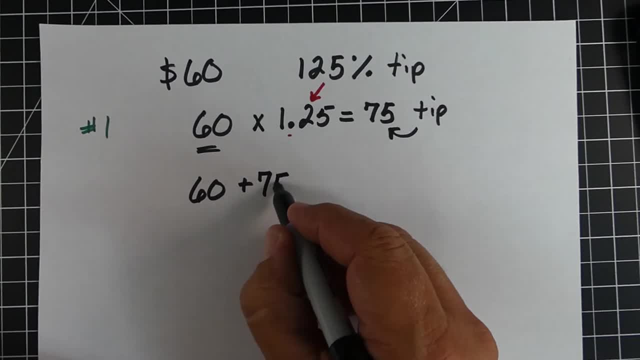 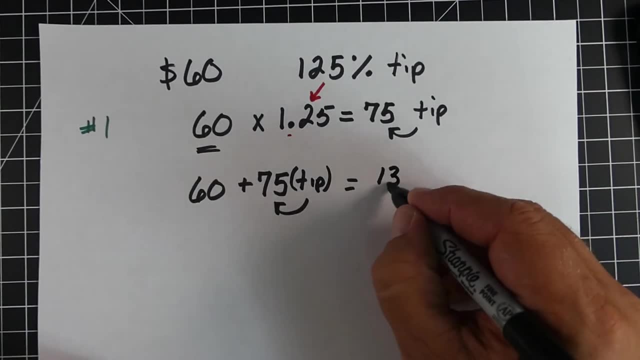 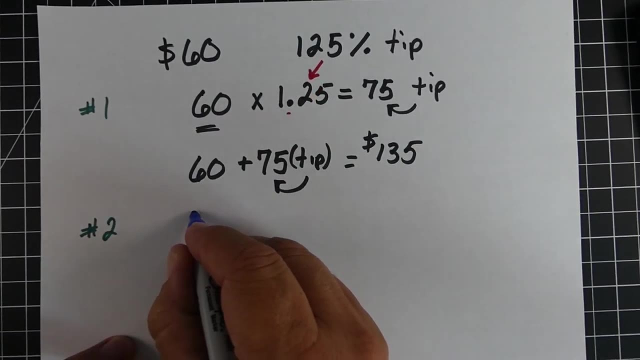 a tip To find the total cost. we take the $60 for the meal plus the $75, which is the amount of tip, and we add those two together. we're going to get $135.. That's our cost with the tip. Now, using method two, we're going to take the $60 again. 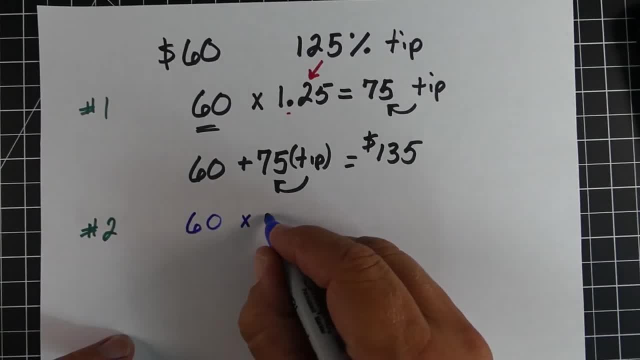 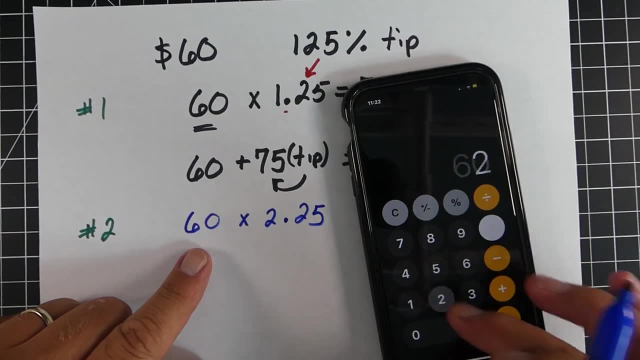 but this time we're going to add or we're going to multiply- excuse me- 2.25. And when we do that we should end up with the same answer. So let's kind of double check our work 60 times 2.25. And sure enough, we're getting $135, just like we did with the first.